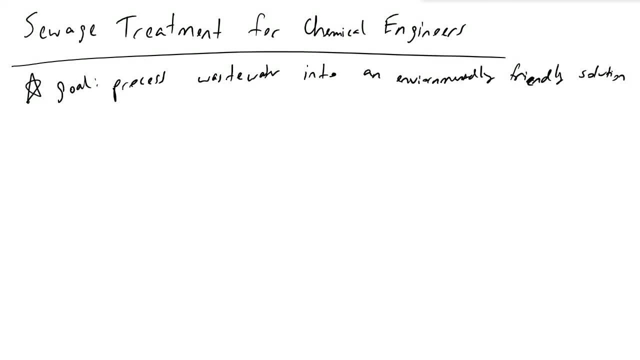 Sewage treatment is arguably one of the most important aspects of modern life. What makes the world we live in today so much different from what people used to live in in the mid-1600s in France, for instance, where you had outbreaks of cholera and all these other terrible things? 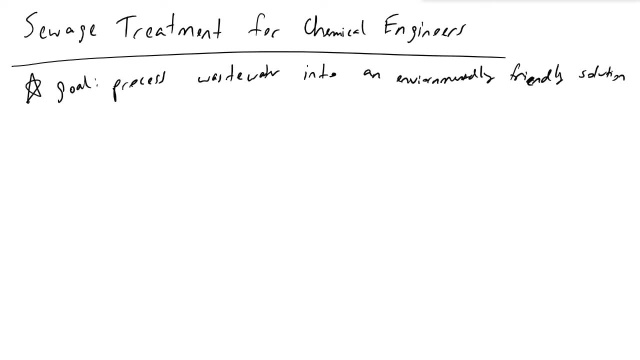 because people didn't have proper ways of disposing of their wastewater, And so in this video, what I'd like to do is go over how chemical engineers are playing integral roles in how society today can actually process wastewater into environmentally friendly solutions, And so it's a pretty cool process, And if you ever get a chance to, I highly recommend visiting your local. 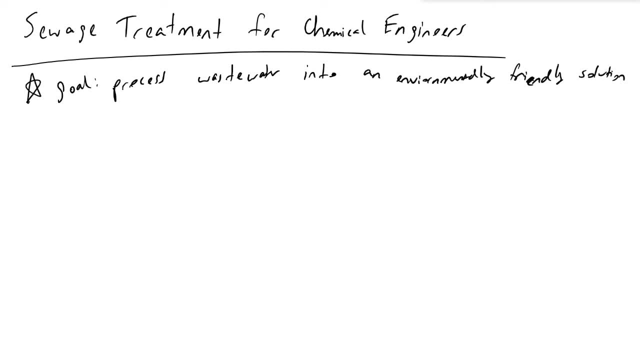 county's sanitary district and just getting a feel for the scale and the size of everything. It's really cool stuff, And if you're a chemical engineer, you're going to see a lot of what you've learned in the classroom applied to the real world. And so the first thing that 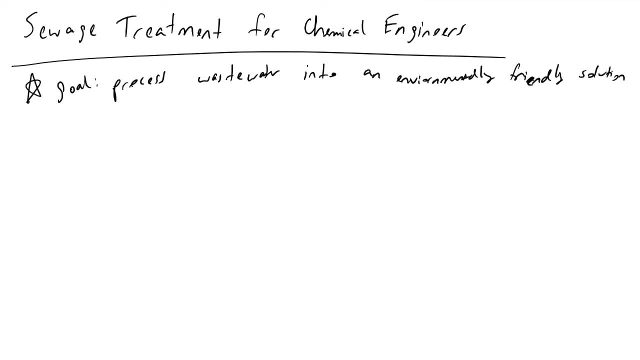 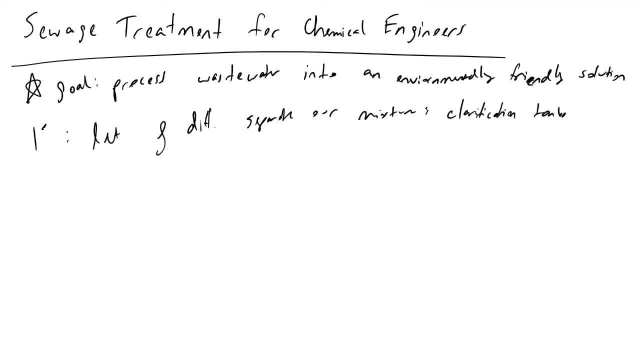 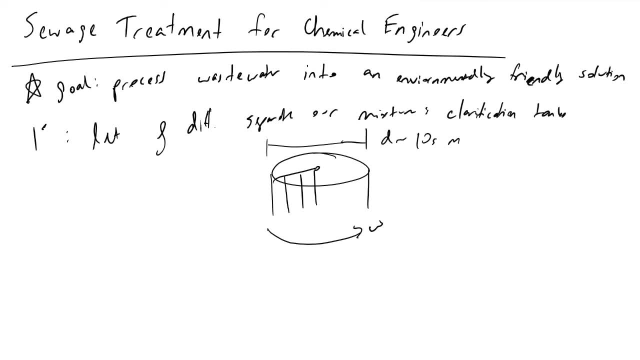 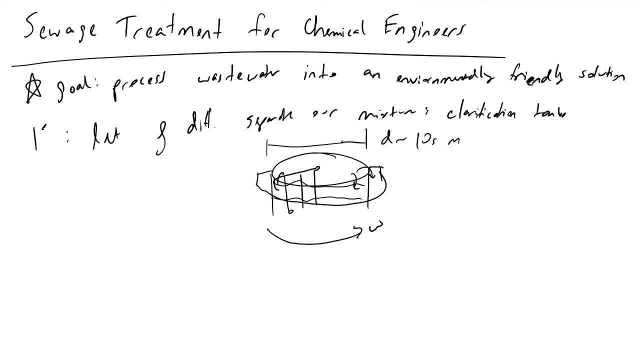 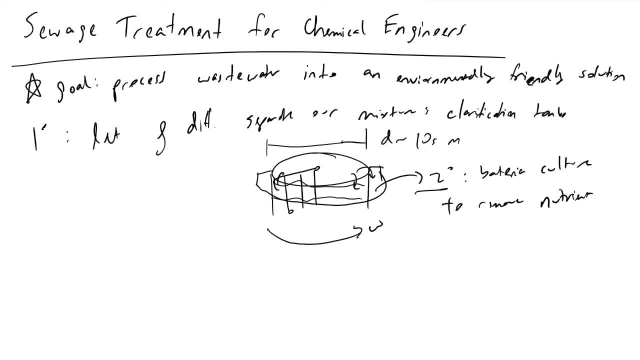 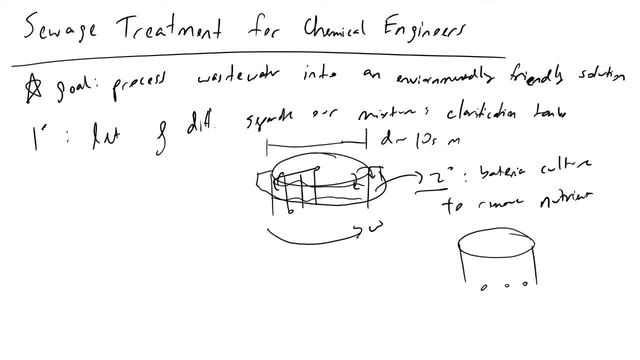 are. you can almost think of it as: And at the bottom we're going to have, we're going to need to bubble oxygen through. So we want to keep O2 levels high inside of these tanks where we have the bacteria processing the wastewater. And the reason for that is because the bacteria needs to perform cellular respiration and therefore they need O2 to do that, And so once the bacteria have removed as many of the nutrients as they can from the 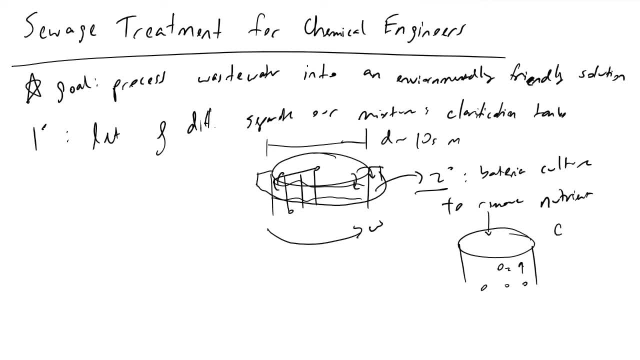 our solution. I'll define some variable CS, for instance for the substrate levels. we're going to decrease the levels of substrate, So algae can't use it. In addition to this, there are some sanitary districts that will try out different strains of bacteria to consume the nitrates and other nutrients that algae are known to consume in order to 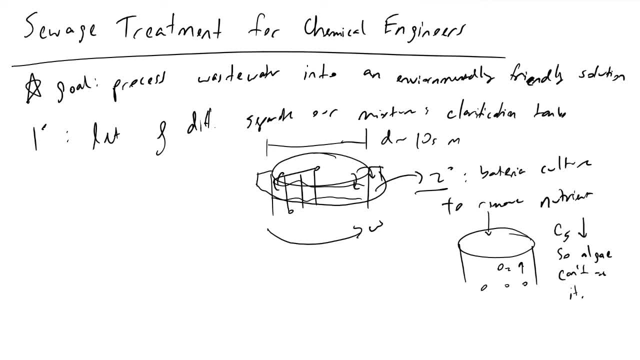 proliferate in local ecosystems, And so that's a big part of this, too- is you'll have technicians and labs periodically doing samples to make sure that your product is will be environmentally friendly. at the end of the day, The next thing that happens after the bacteria have consumed all the nutrients is we will hit our solution with very intense UV lights, and we're processing tens of thousands of 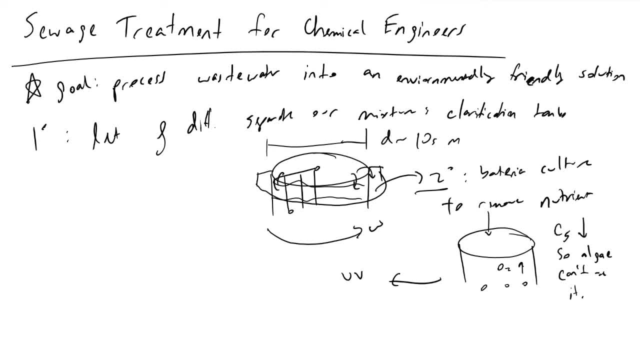 gallons of this every hour, And so what the UV light will do is it will kill all the life that is present. so the bacteria included in our solution, And after it does that, the next step is to again kind of aerate the water, because we need to keep O2 levels at a particular level, such 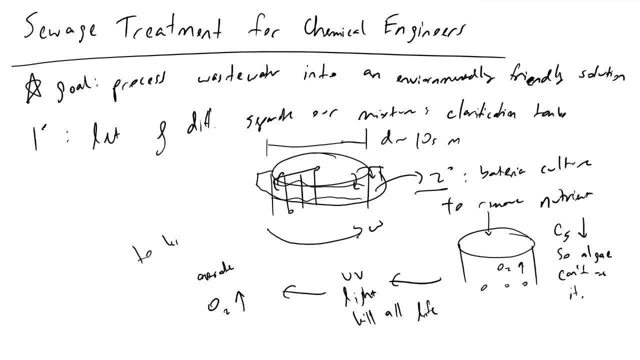 that we don't kill those nutrients, um to not kill- sorry, to not kill- fish. So if we took the water at this point and dumped it into the bay, the problem we'd run into is a lot of fish would die because, um, there's so low oxygen. 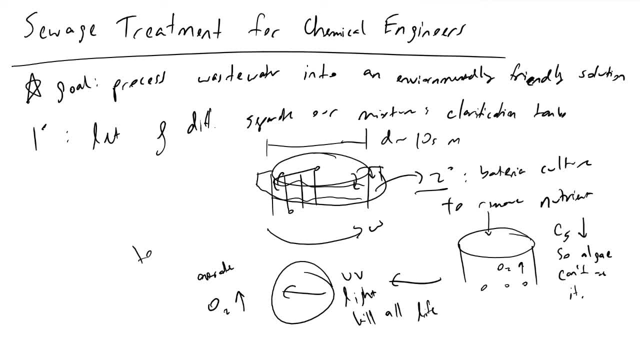 concentrations that, uh, the fish can't live in those kinds of environments because they can't perform cellular respiration either. Um and so after this point, uh, it actually will go out to the bay, for instance. And the thing to ask at this point is: how do you do that? And so we have